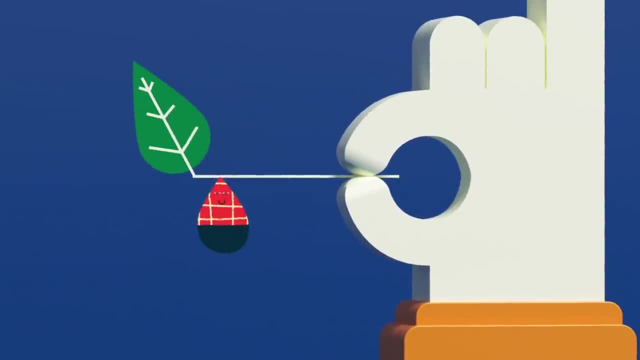 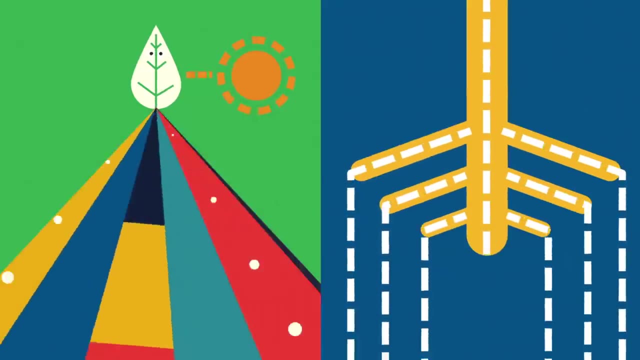 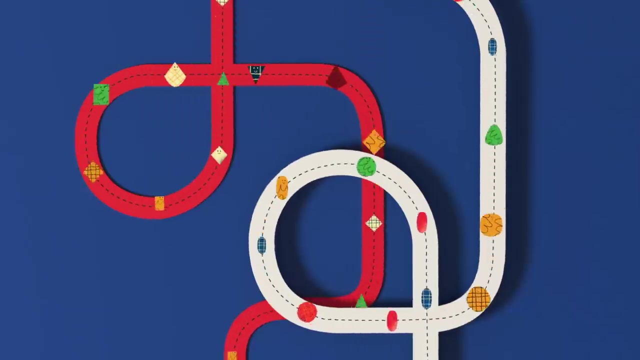 It all comes down to sap. In order for trees to grow, they need to bring sugars obtained from photosynthesis and nutrients brought in through the root system to wherever growth is happening. And just like blood circulates in the human body, trees are designed to circulate two kinds of sap throughout their bodies. 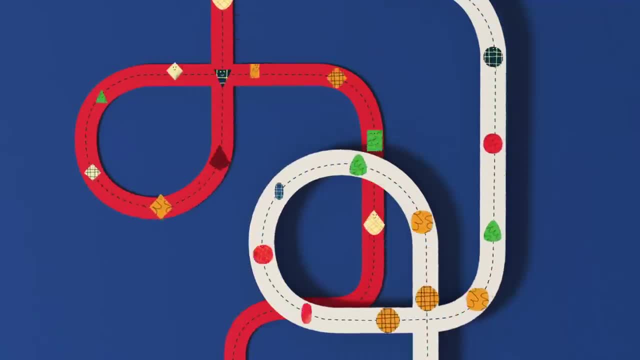 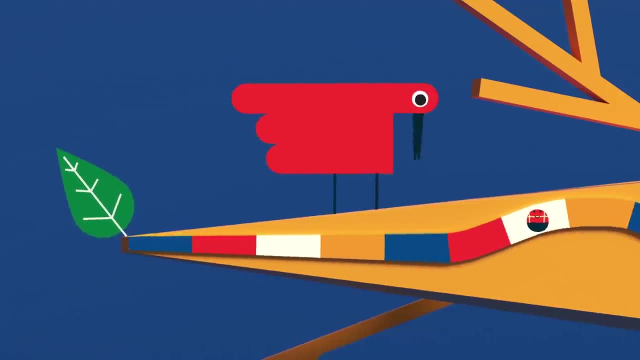 carrying all the substances a tree's cells need to live. The first is phloem sap, Containing the sugars generated in leaves during photosynthesis. phloem sap is thick like honey and flows down the plant's phloem tissue. 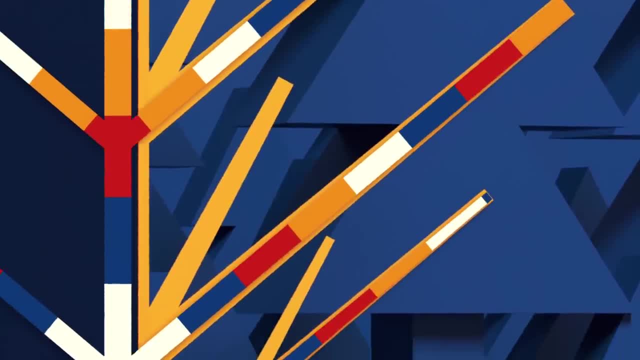 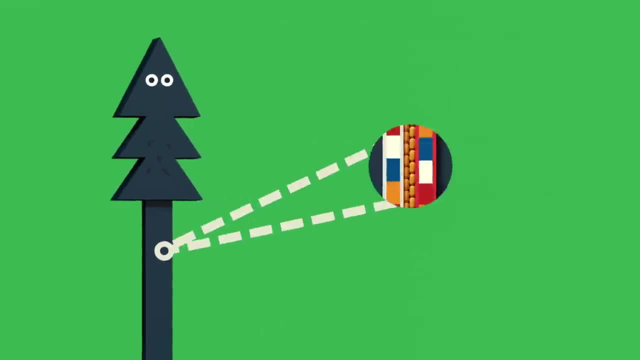 to distribute sugar throughout the tree. By the end of its journey, the phloem sap has thinned into a watery substance pooling at the base of the tree. Right beside the phloem is the tree's other tissue type, the xylem. 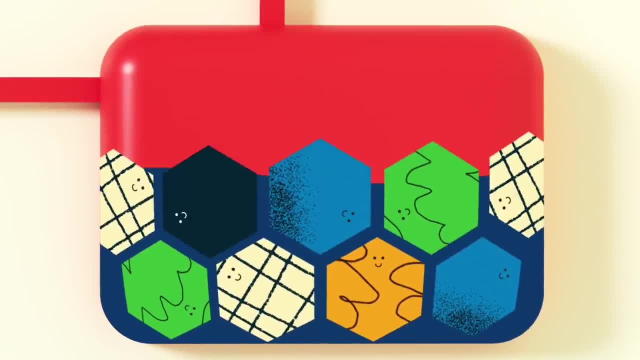 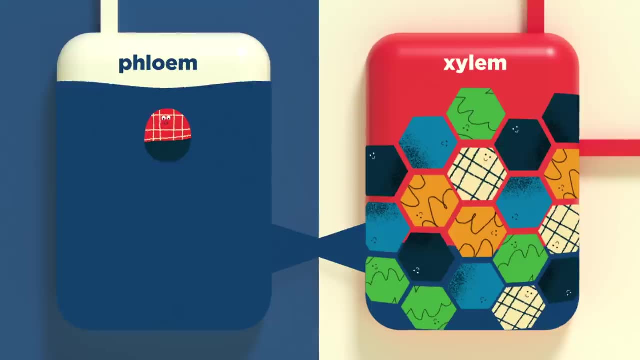 This tissue is packed with nutrients and ions like calcium, potassium and iron, which the tree has absorbed through its roots. Here at the tree's base. there are more of these particles in one tissue than the other, so the water from the phloem sap is absorbed into the xylem. 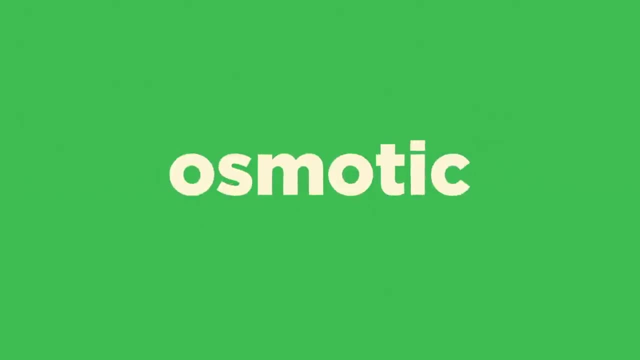 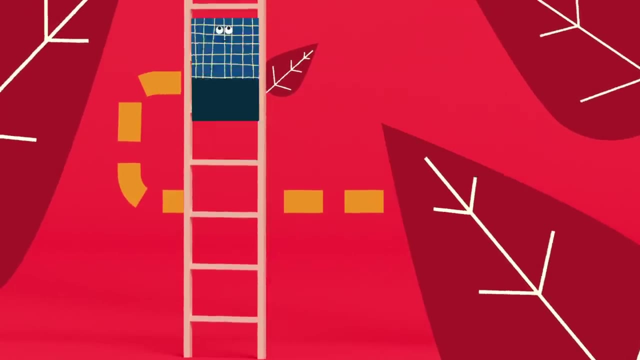 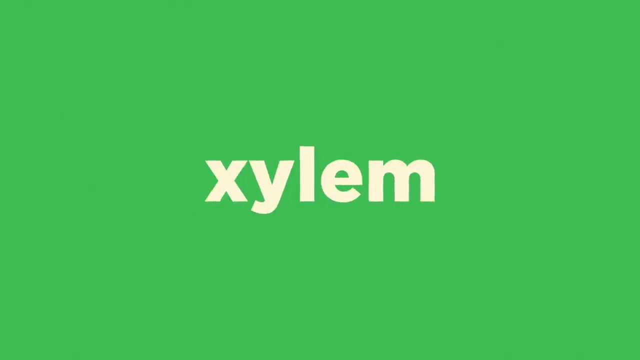 to correct the balance. This process, called osmotic movement, creates nutrient-rich xylem sap which will then travel up the trunk to spread those nutrients through the tree. But this journey faces a formidable obstacle— gravity To accomplish this Herculean task. 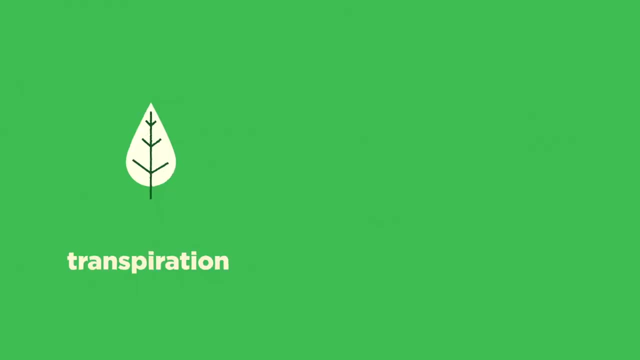 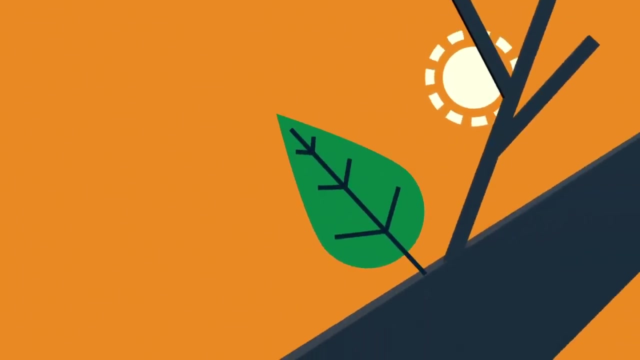 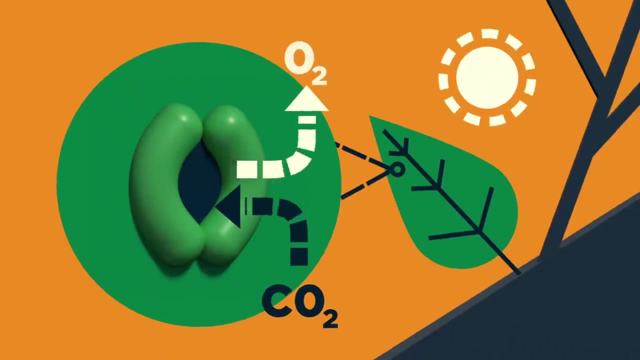 the xylem relies on three forces— transpiration, capillary action and root pressure. As part of photosynthesis, leaves open and close pores called stomata. These openings allow oxygen and carbon dioxide in and out of the leaf, but they also create an opening. 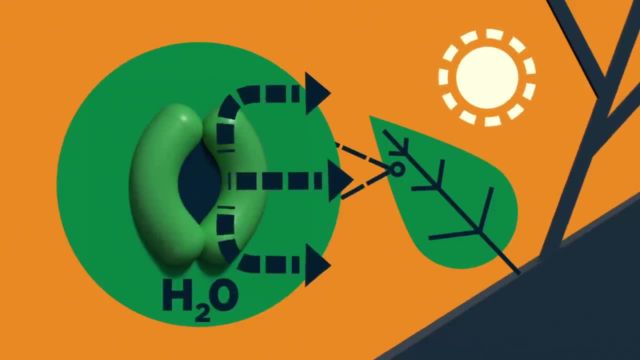 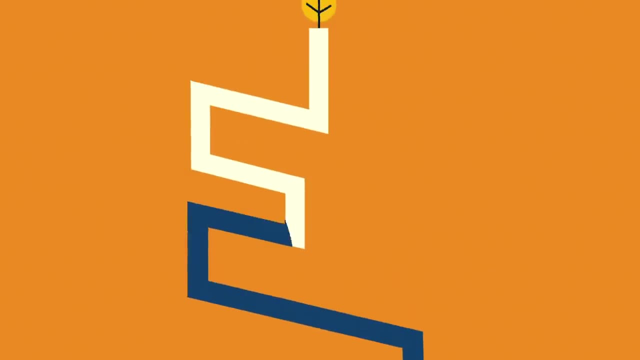 through which water evaporates. This evaporation, called transpiration, creates negative pressure in the xylem pulling watery xylem sap up the tree. This pull is aided by a fundamental property of water called capillary action In narrow tubes. 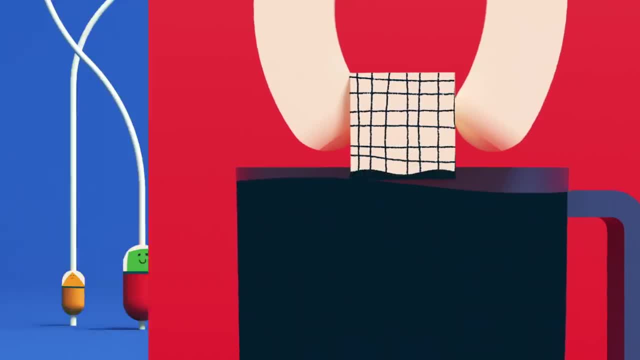 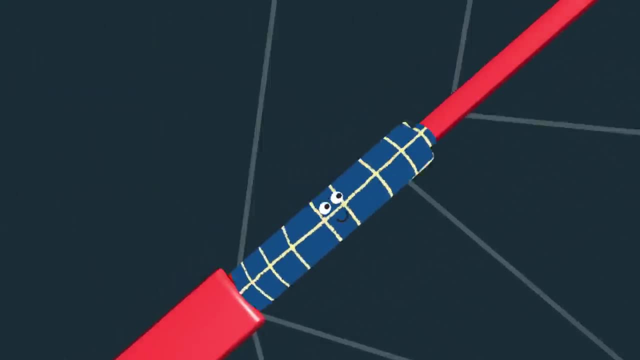 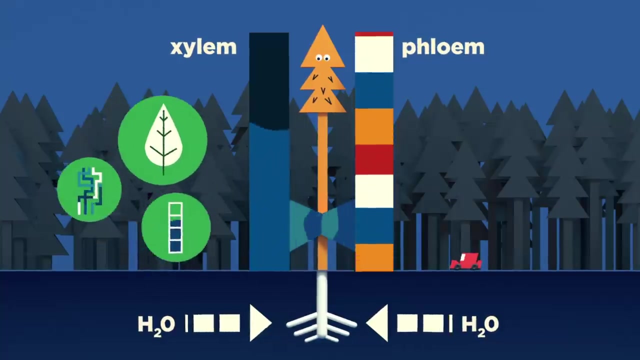 the attraction between water molecules and the adhesive forces between the water and its environment can beat out gravity. This capillary motion is in full effect in xylem filaments thinner than human hair, And where these two forces pull the sap, the osmotic movement at the tree's base.